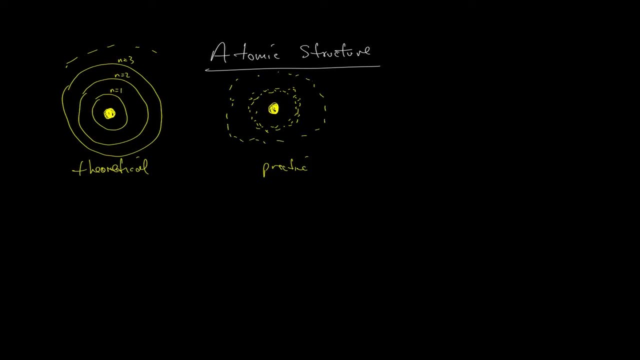 Again, that's got a whole list of possible positions about where that electron could be. Well, there are some statistical analyses to help us here, which gives us the simplistic model here. So we can just say, okay, shell 1,, 2,, 3,, 4,, etc. 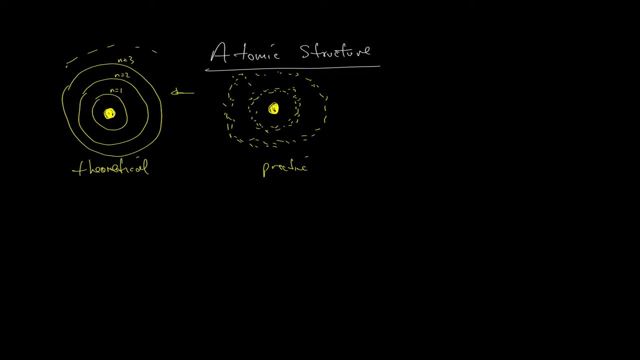 And essentially, if an electron- let me get the colour of an electron- light blue, like so, So electrons out there- it's going to have a higher energy level than as if it was here. So the higher up you go, the more energy the electron has. Okay. 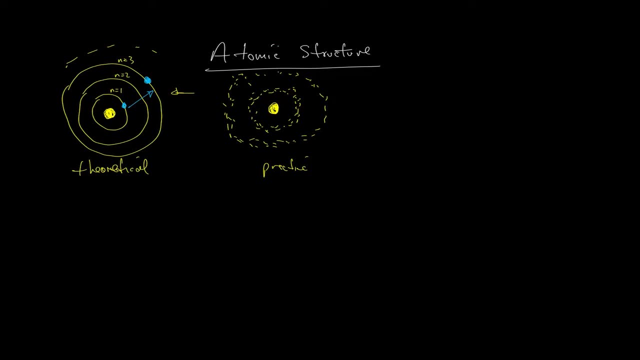 Now then? so what do we do about these actual shells themselves? We have a shell, We give it a number, n, Okay, And normally we go up to 5, and we then tend to stop because things get a little bit unpredictable and uncertain after this idea of shell number 5.. 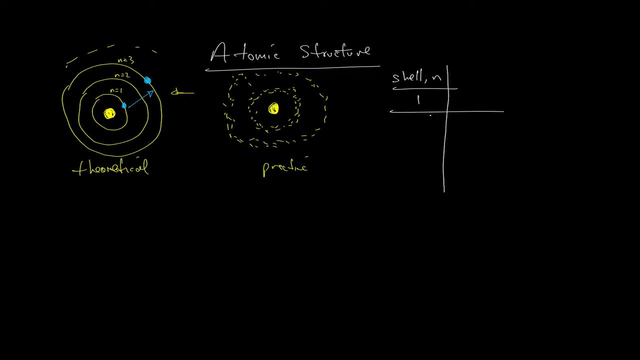 Okay, So we're going to start off with 1,, 2,, 3, 4, 5.. And then we go on with 1,, 2,, 3,, 4, 5.. Like so Okay. 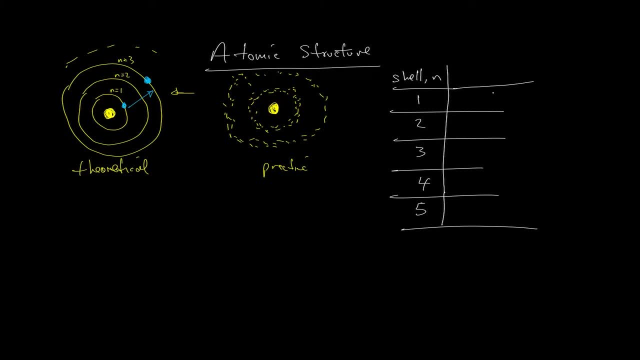 And what I would like to do is to put in well a basic algorithm that we use in terms of the maximum number, So maximum number of electrons We call electrons E. shall we Maximum the electrons? it's going to be equal to two times the n value squared. okay, so the n values on the 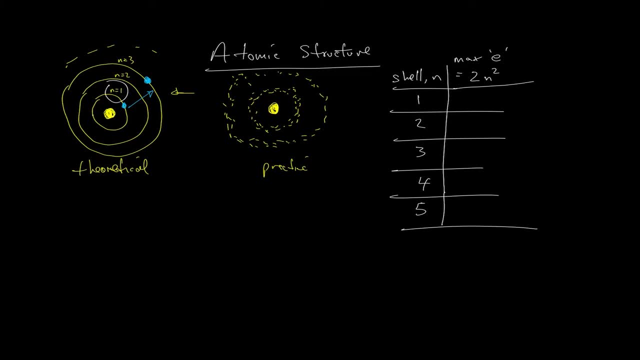 left here. so shell one which is over here, that one, we can say: well, one squared is one, two ones are two. if a second shell. so two squared gives you four, two, fours give you eight. third shell: three squared gives you nine. two, nines are 18.. now you see where we're going with this. okay, fourth shell. 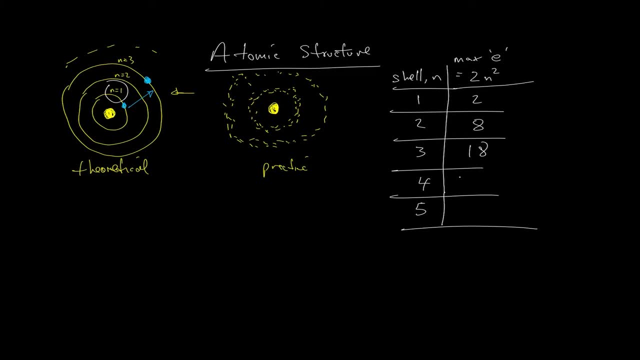 four squared gets you 16 to 16 to 32, and the final one we're going to deal with is the fifth shell. five squared is 25, 225 is 50.. so theoretically, that's the maximum number of uh electrons that can reside in any particular. 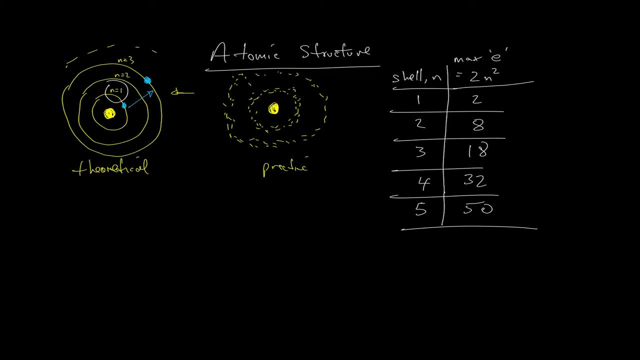 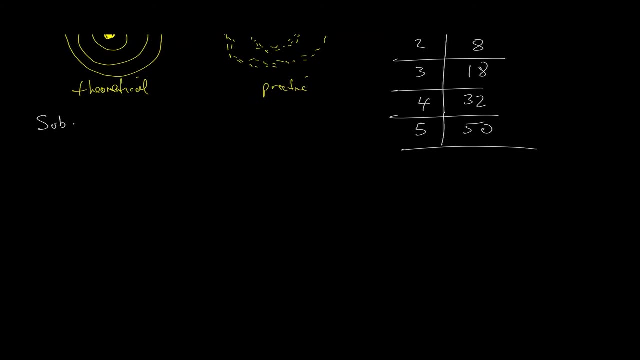 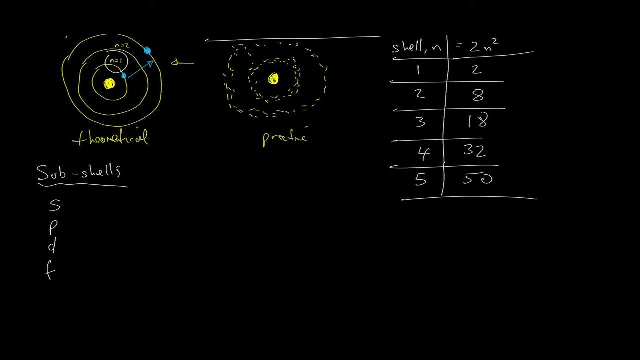 shell. interestingly, we also have sub shells, so sub shells. let's bring this back up so you can see these shell numbers there. okay, sub shells. uh, historically there are the tense before. so we have- i'm not going to go through why to be give them these letters, but they just were historically okay. SPDF: we like to. 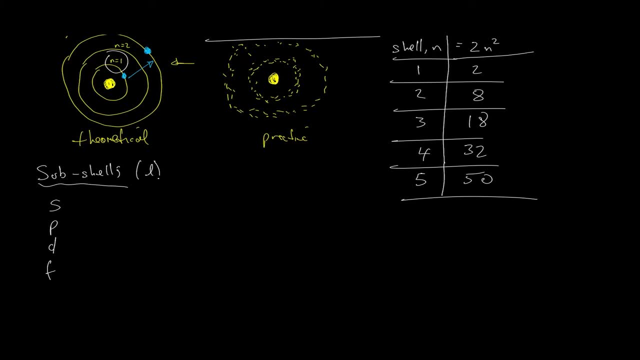 give them what we call an L number. so L, we're going to say this L number, this no. so this is moving out, if you like. so in here we are going to have one, here we'll have two sub shells, here we'll have three sub shells, etc. okay, so the 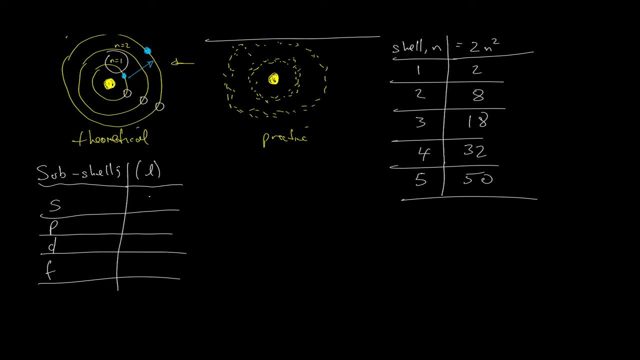 first sub shells, I was s, then P, then D, then F. but to make it a bit more scientific, we use the numbers for L, 0, 1, 2 and 3, and we also have another algorithm here. so the maximum number of electrons in a sub shell is actually equal to 2 lots of 2l plus 1. 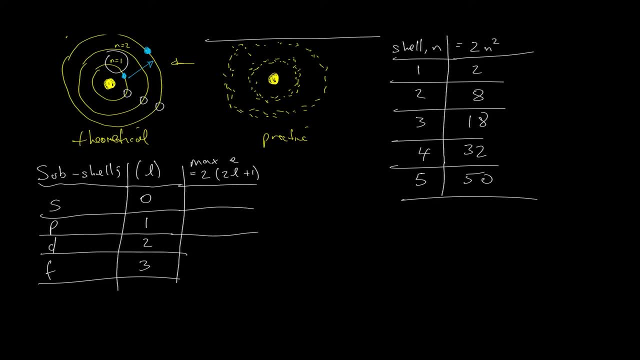 okay, so we can work out how many electrons are going to be in the s shell. so we just s is 0, of course, and that's a number of electrons in a sub shell. so we can work out how many electrons are going to be in the s shell. so we just s is 0, of course, and that's a. 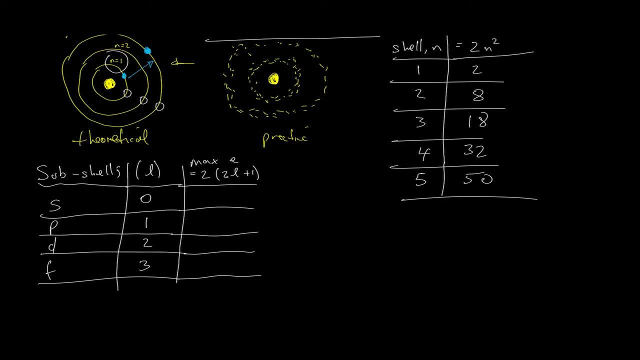 number of electrons in a sub shell, so we can work out how many electrons are going to be in the s shell. so we just: s is 0, of course, and that's a. so replace L with 0. 2 zeros is nothing. there's one in brackets 2 times 1. 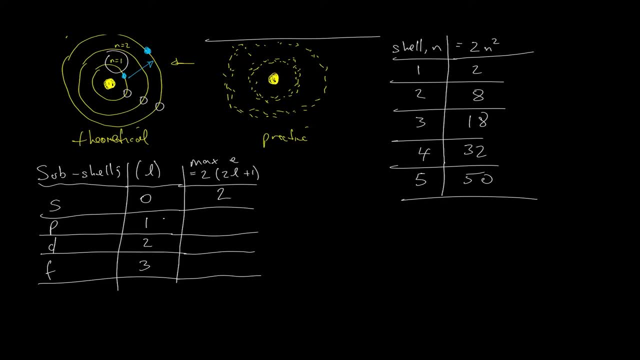 so replace L with 0. 2 zeros is nothing. there's one in brackets 2 times 1, so replace L with 0, 2 zeros is nothing. there's one in brackets. 2 times 1 gives us 2. okay, here our L value for P. 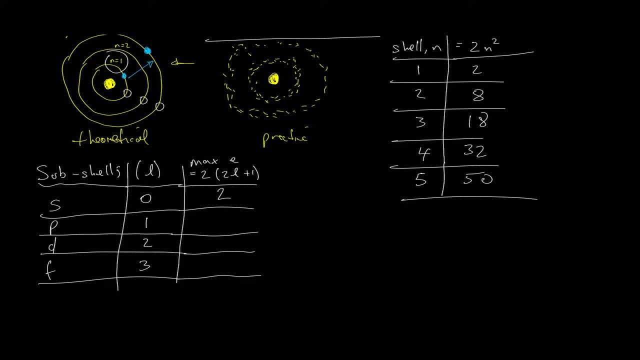 gives us 2. okay, here, our L value for P gives us 2. okay, here, our L value for P is one, so two ones are two plus one is is one, so two ones are two plus one is is one, so two ones are two plus one is three, two, threes are six. okay, here the L. 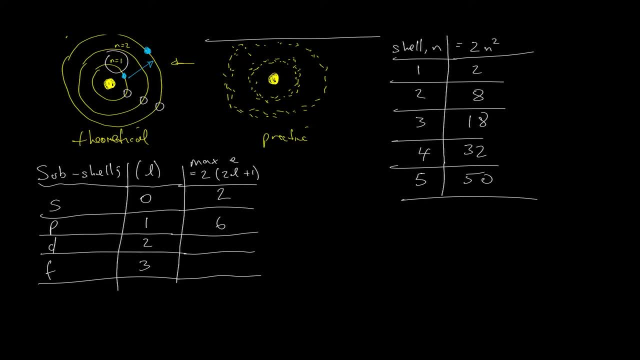 three, two, threes are six. okay here the L. three, two, threes are six. okay here the L. value for D is two, so two. twos of four. value for D is two, so two. twos of four. value for D is two, so two. twos of four plus one is five. two, fives are ten okay. 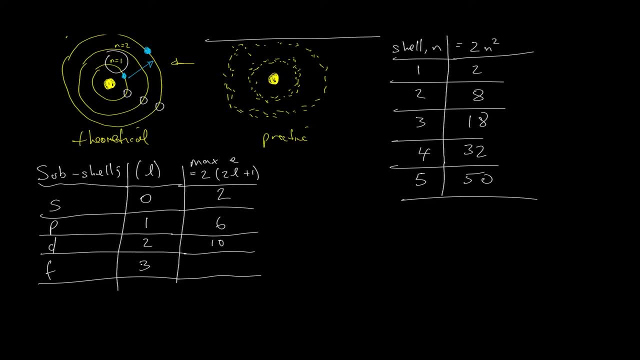 plus one is five. two fives are ten, okay. plus one is five. two fives are ten, okay. and finally the F shell L is three here, and finally the F shell L is three here and finally the F shell L is three here. so two, threes are six plus one is seven. 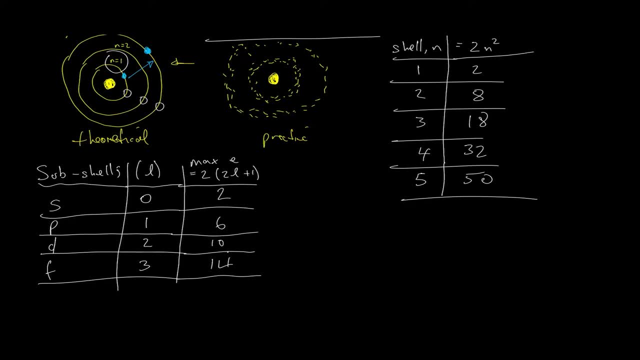 so two threes are six plus one is seven. so two threes are six plus one is seven, two sevens or 14, and you'll notice of two sevens or 14, and you'll notice of two sevens or 14, and you'll notice, of course, that these things are moving up. 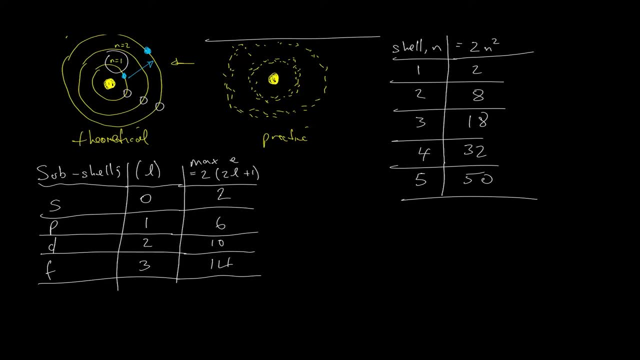 course that these things are moving up, course that these things are moving up in force. okay, you start me to add four in force. okay, you start me to add four in force. okay, you start me to add four, add four, add four, right. so now I'm going. 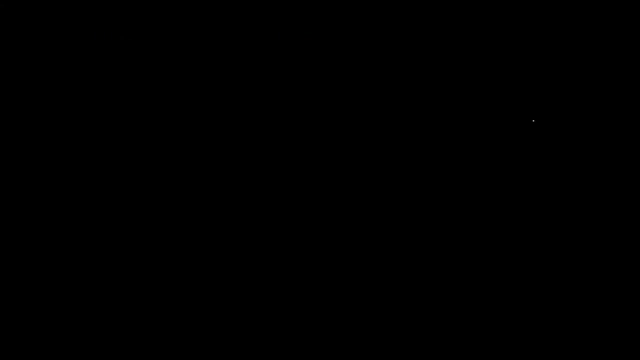 add four, add four, right. so now I'm going: add four, add four, right. so now I'm going to get to the nitty-gritty, and I want to get to the nitty-gritty, and I want to get to the nitty-gritty and I want to talk about the periodic table and 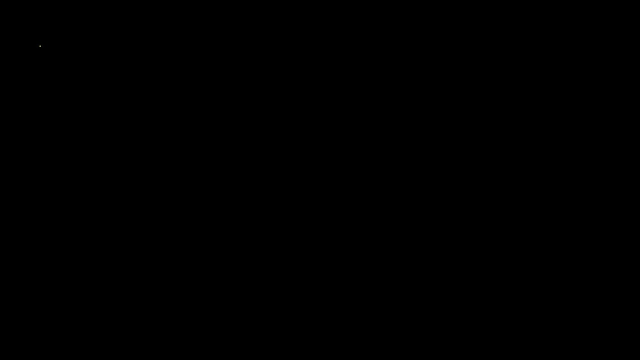 to talk about the periodic table and to talk about the periodic table and some notation that we use, and I would some notation that we use and I would some notation that we use and I would like to mention possibly the first maybe. like to mention possibly the first maybe. 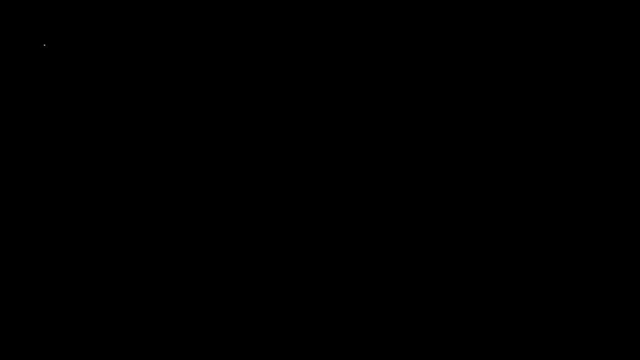 like to mention possibly the first, maybe ten or eleven elements. okay, to show you ten or eleven elements. okay, to show you ten or eleven elements. okay, to show you how the shells in the in the lower, how the shells in the in the lower, how the shells in the in the lower elements are populated. okay, so I'm good. 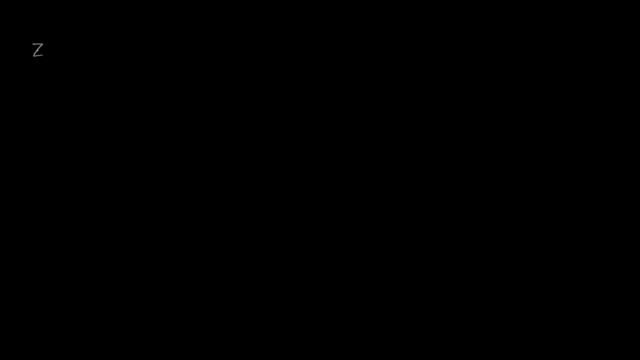 elements are populated okay, so I'm good. elements are populated okay, so I'm good. first of all, put some headings in. so first of all put some headings in. so first of all put some headings in. so I'm going to have a Zed number of the. 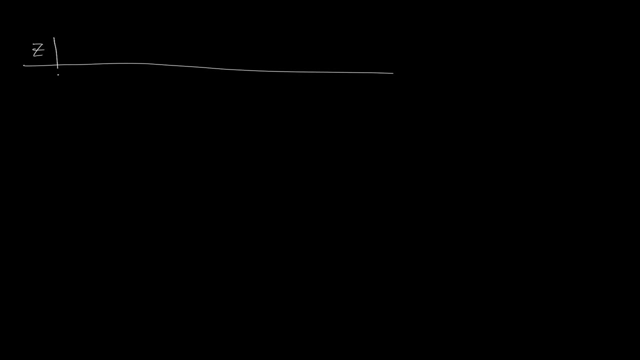 I'm going to have a Zed number of the. I'm going to have a Zed number of the atomic number, which is that you see the atomic number, which is that you see the atomic number, which is that you see the number of protons in the elements. then 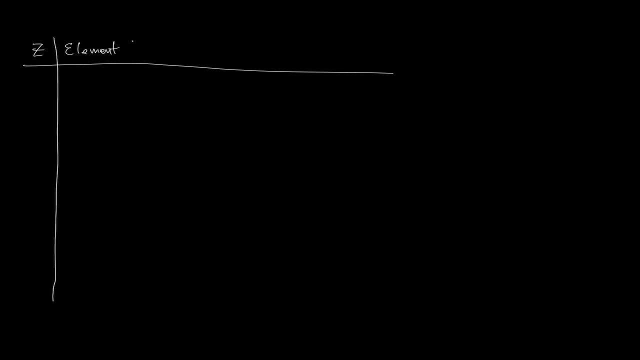 number of protons in the elements. then number of protons in the elements. then name the element for you. name the element for you. name the element for you. I'm also going to give you its symbol. I'm also going to give you its symbol. I'm also going to give you its symbol, and this is the important bit, we're. 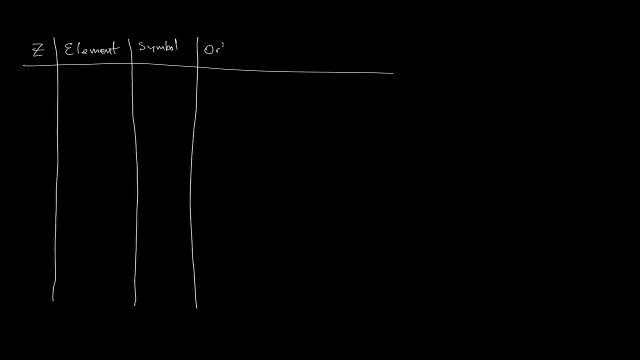 and this is the important bit- we're- and this is the important bit we're going to going to, going to in, in, in- indicate the orbital notation, in other indicate the orbital notation, in other indicate the orbital notation. in other words, we're going to describe how many. 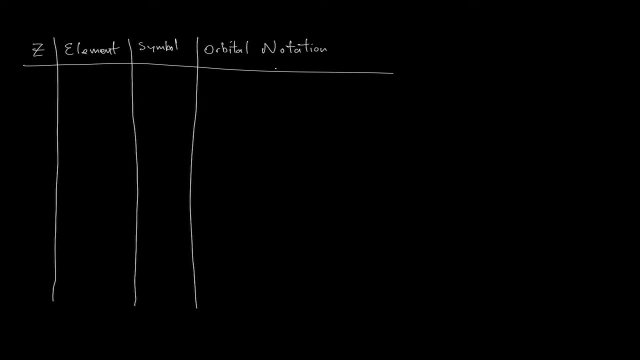 words. we're going to describe how many words. we're going to describe how many electrons are in the main shells and the electrons are in the main shells. and the electrons are in the main shells and the sub shells. okay, so maybe I could draw sub shells. okay, so maybe I could draw. 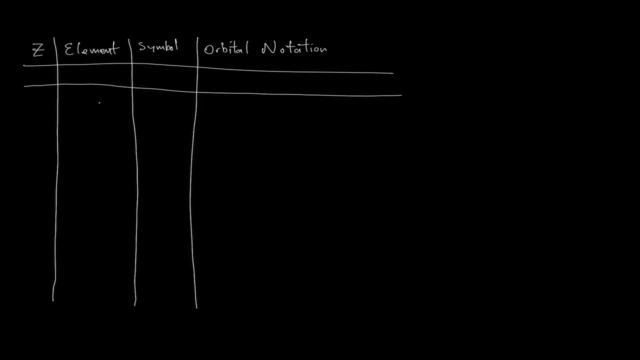 sub shells. okay, so maybe I could draw the table first. so I don't want to run the table first. so I don't want to run the table first, so I don't want to run out of room, out of room, out of room, to, to, to, to. 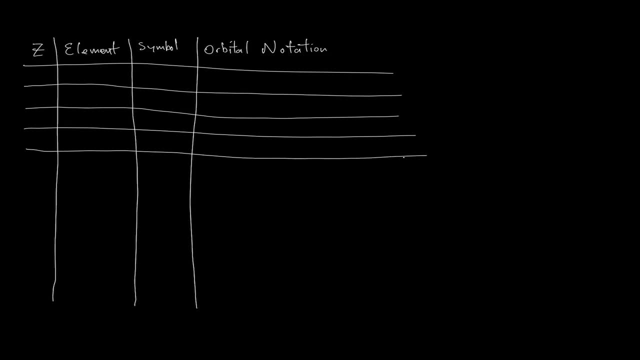 to to to three, three, three, four, four, four, five, five, five, six, six, six, seven, seven, seven, eight, eight, eight, nine, nine, nine, ten will be room for 11. okay, so ten will be room for 11. okay, so ten will be room for 11. okay, so maybe we should change color now. 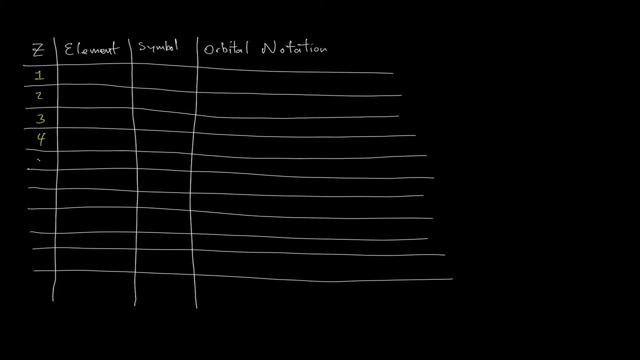 maybe we should change color now. maybe we should change color now: one, two, one, two, one, two, three, three, three, three, four, three, four, five, six, seven, eight, nine, ten, eleven protons, etc. okay, I'm going. three, four, five, six, seven, eight, nine, ten, eleven protons, etc. okay, I'm going. 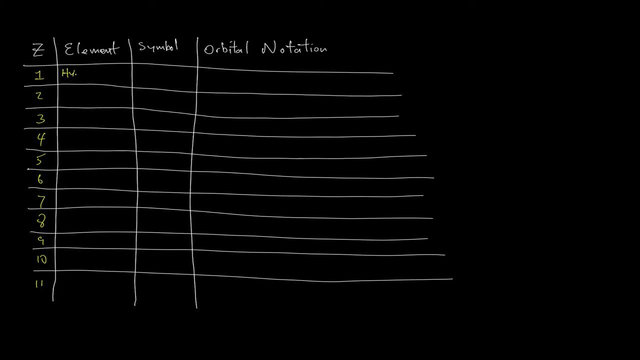 three, four, five, six, seven, eight, nine, ten, eleven protons, etc. okay, I'm going to start with hydrogen hydrogen, to start with hydrogen hydrogen. to start with hydrogen hydrogen. symbol is H and well, that number gives it away. symbol is H and well, that number gives it away. 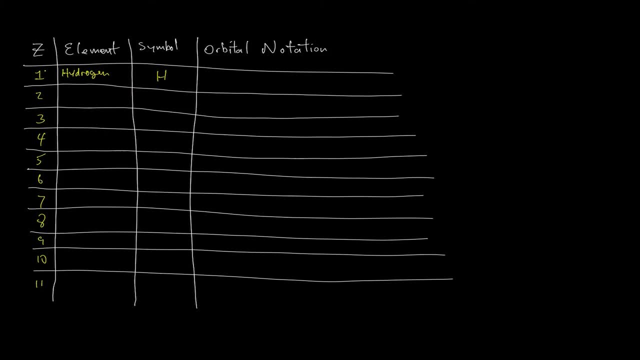 symbol is H, and well, that number gives it away. so we're looking at the number of. so we're looking at the number of. so we're looking at the number of electrons. now, so this is a neutral electrons. now, so this is a neutral electrons. now, so this is a neutral hydrogen with the 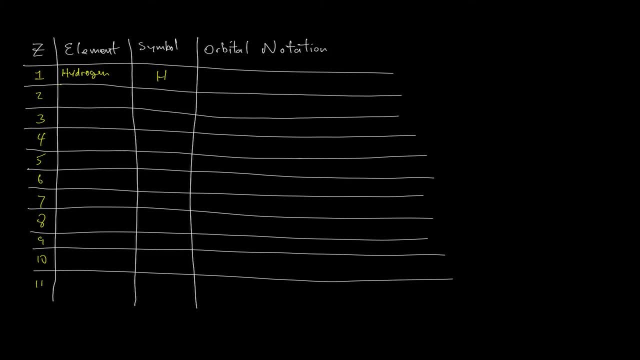 hydrogen with the, hydrogen with the. so we're not talking about an ion in any so. we're not talking about an ion in any so. we're not talking about an ion in any way. there's no char net charge is zero. way, there's no char net charge is zero. 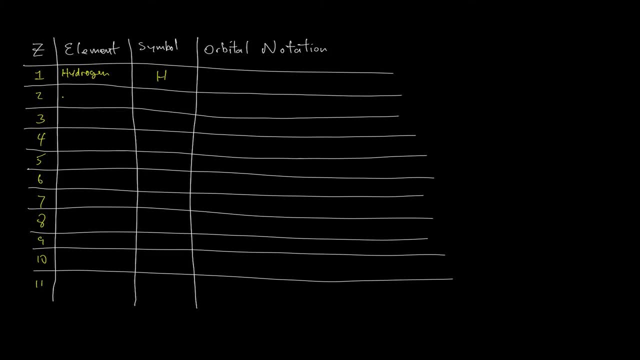 way. there's no char. net charge is zero. but we do have one orbiting electron, and, but we do have one orbiting electron, and, but we do have one orbiting electron and that electron predictably sits in shell. that electron predictably sits in shell. that electron predictably sits in shell number one, which is closest to the 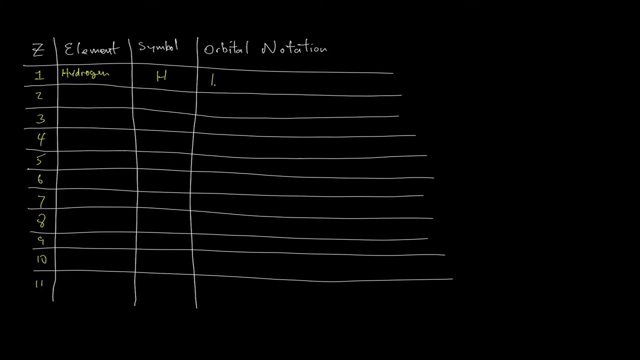 number one which is closest to the number one which is closest to the nucleus, then you have to deal with nucleus, then you have to deal with nucleus, then you have to deal with subshells. well, the first one only has subshells. well, the first one only has. 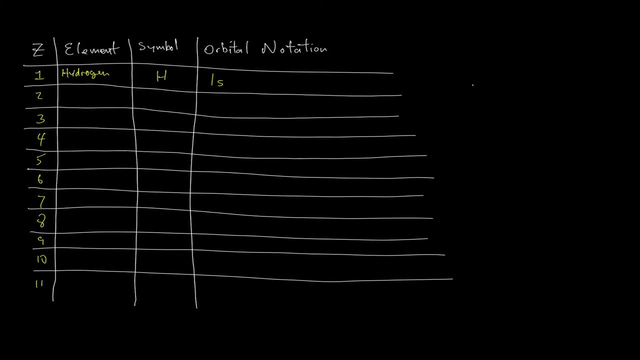 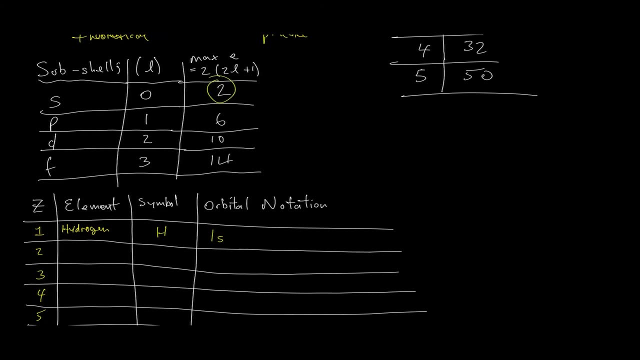 subshells. well, the first one only has the S shell, and we only have one, the S shell, and we only have one, the S shell, and we only have one, electrons. okay, well, it's just one s to electrons. okay, well, it's just one s to. 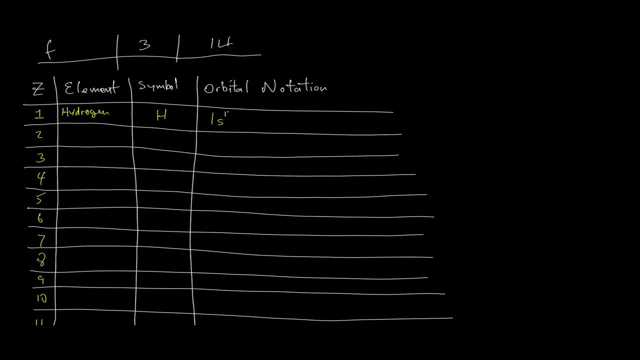 electrons. okay, well, it's just one s to the power one. so all these powers and the power one. so all these powers and the power one. so all these powers, and indicating: here is one they should be indicating. here is one they should be indicating, here is one. they should be matching this number here: the total when. 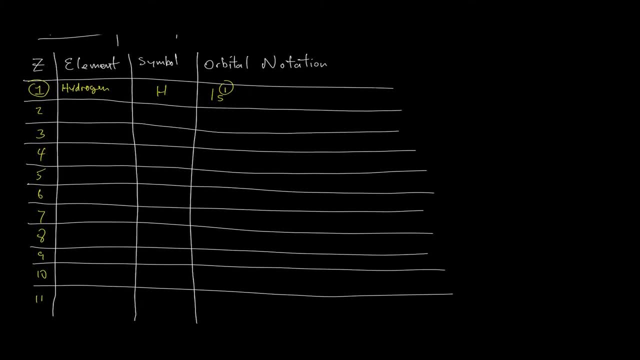 matching this number, here the total when. matching this number, here the total when you add them all up. okay, right, so now you add them all up. okay, right, so now you add them all up. okay, right, so now I'm going to move on to the second. I'm going to move on to the second. 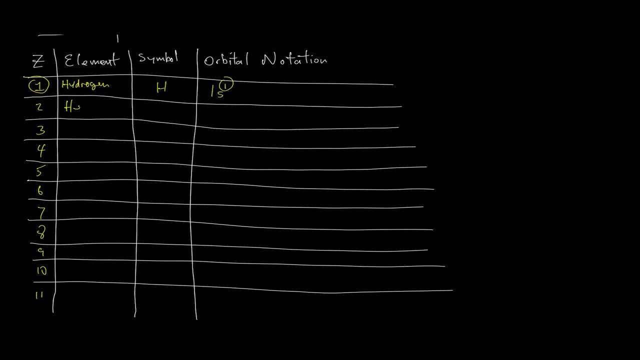 I'm going to move on to the second element in the periodic table, which is element in the periodic table, which is element in the periodic table, which is helium, oops, helium, helium, oops, helium, helium, oops, helium. symbol H e. this is similar to hydrogen. symbol H e. this is similar to hydrogen. 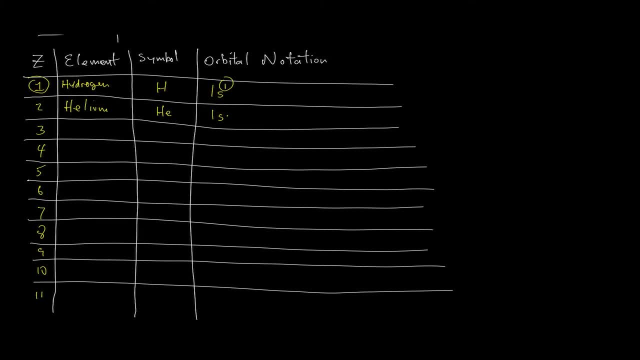 symbol H e. this is similar to hydrogen, except rather than one electron in the. except rather than one electron in the. except rather than one electron in the 1s shell. it has two. okay, the maximum 1s shell. it has two. okay, the maximum 1s shell. it has two. okay, the maximum allowed is two in this sub shell anyway. 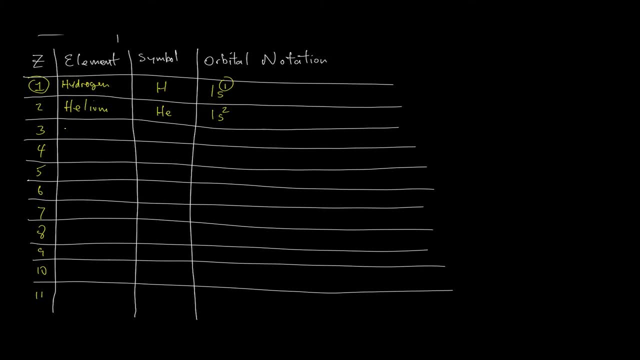 allowed is two in this sub shell anyway. allowed is two in this sub shell anyway. the third elements. we're going to be the third elements. we're going to be the third elements we're going to be looking at is lithium, those who know. looking at is lithium, those who know. 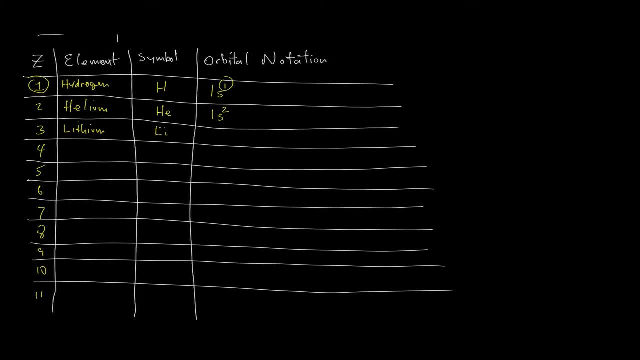 looking at is lithium, those who know your periodic table, your periodic table, your periodic table li, so that one has that in a shell fully li, so that one has that in a shell fully li, so that one has that in a shell fully populated, then it has to go, maybe I. populated, then it has to go. maybe I populated, then it has to go. maybe I could leave the gap here normally. we could leave the gap here. normally, we could leave the gap here. normally, we don't leave the gap, for I'm going to don't leave the gap, for I'm going to. 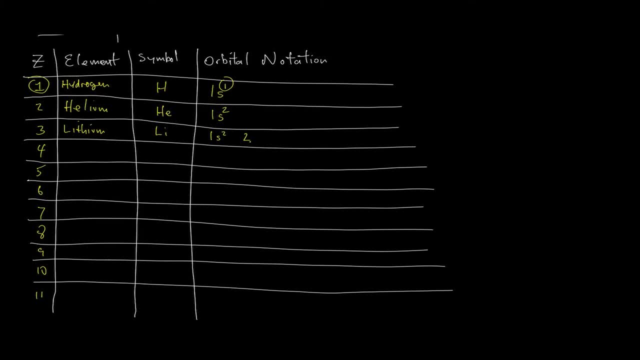 don't leave the gap, for I'm going to leave one for you, just to indicate that. leave one for you, just to indicate that. leave one for you, just to indicate that we've moved to a different shell 2s to. we've moved to a different shell 2s to. 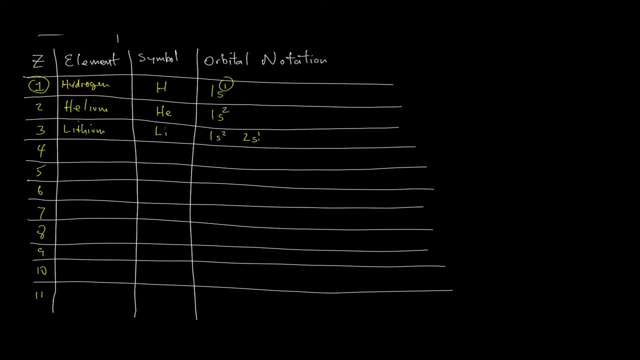 we've moved to a different shell. 2s to the one. so we're always moving one, two the one. so we're always moving one, two the one. so we're always moving one, two, three, four, SPD F. okay. so 2s to the one, three, four, SPD F. okay, so 2s to the one. 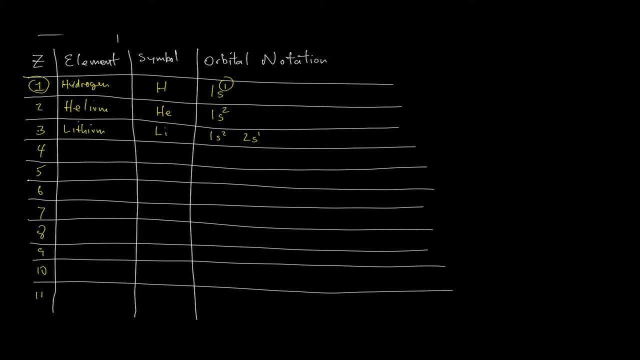 three, four. SPD F: okay, so 2s to the one. and you look at the powers: the two plus and you look at the powers: the two plus. and you look at the powers: the two plus the one gives you this three here, okay. the one gives you this three here, okay. 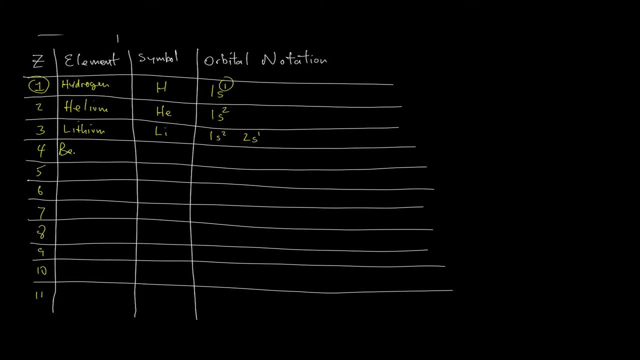 the one gives you this. three here. okay, number four, number four, number four: beryllium in the periodic table. beryllium in the periodic table. beryllium in the periodic table. symbol is be and this is going to have. symbol is be and this is going to have. 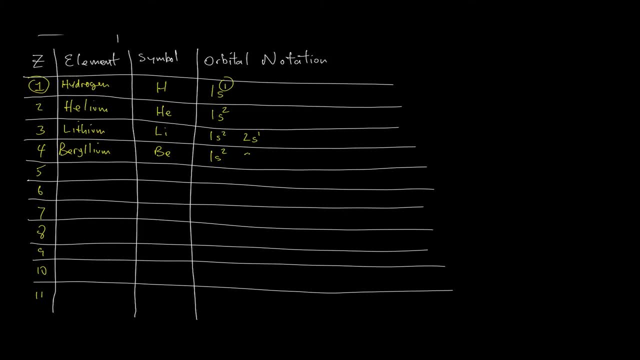 symbol is be, and this is going to have, predictably one s squared, predictably one s squared, predictably one s squared, and then a further one in the two s okay, and then a further one in the two s okay, and then a further one in the two s okay. so two and two. 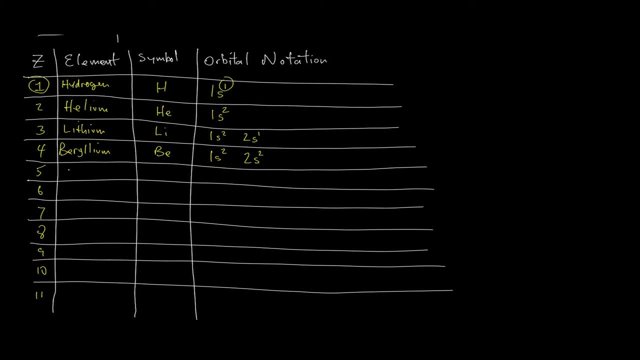 so two and two. so two and two gives you four, gives you four, gives you four. the fifth, the fifth, the fifth is boron symbol is just b for boron. symbol is just b for boron, symbol is just b for boron. this one is one s squared. 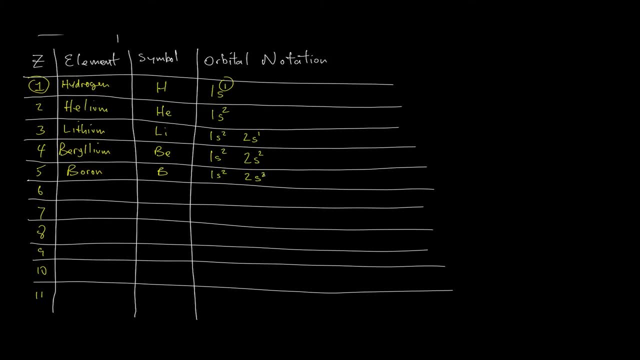 this one is one s squared. this one is one s squared. two, two, two s s s squared, squared, squared. perhaps you can predict the next one. so perhaps you can predict the next one. so perhaps you can predict the next one. so it's spdf, so we're in. 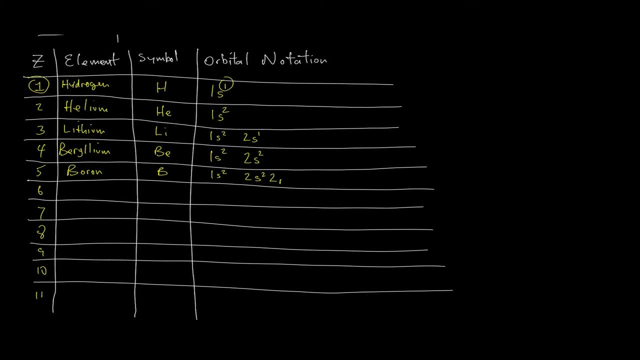 it's spdf, so we're in it's spdf, so we're in the second shell. it needs to be p the second shell. it needs to be p the second shell. it needs to be p to the one. okay, just to remind you, to the one. okay, just to remind you. 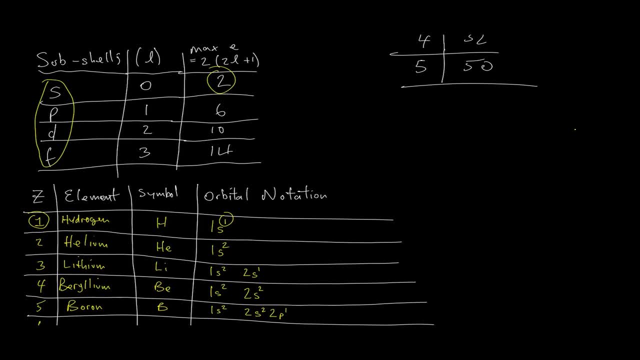 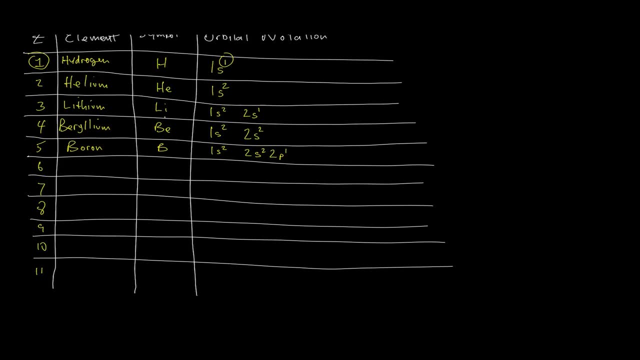 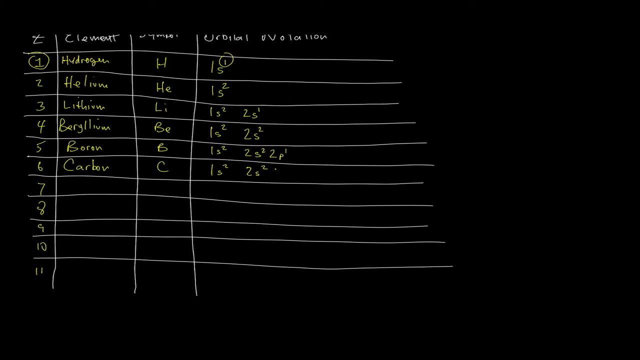 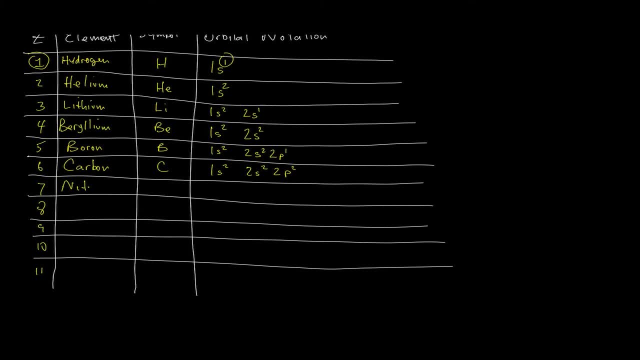 two p two, two, two plus two plus two. two p, two, two, two plus two plus two gives us six, okay, gives us six, okay, gives us six, okay. nitrogen, nitrogen. nitrogen, nitrogen. symbol capital n. symbol capital n. symbol capital n. one s squared one s squared one s squared two s. 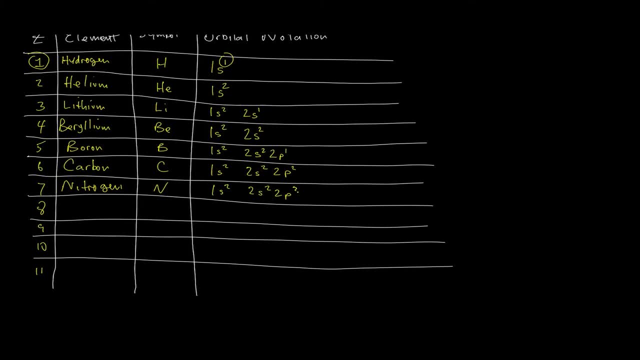 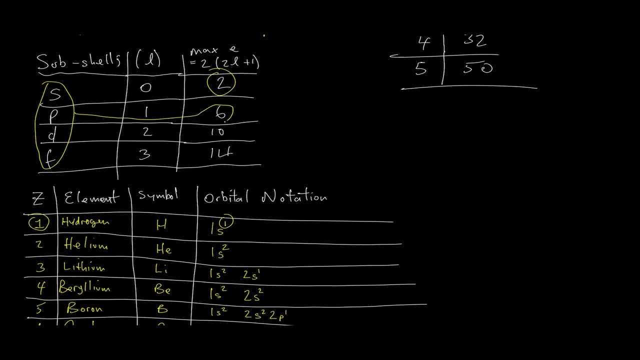 two s squared. two s squared, squared, squared, squared. two p, two p, two p to the three. remember the p to the three, remember the p to the three, remember the p: subshell, subshell, subshell. can go all the way up to six if needed. can go all the way up to six if needed. 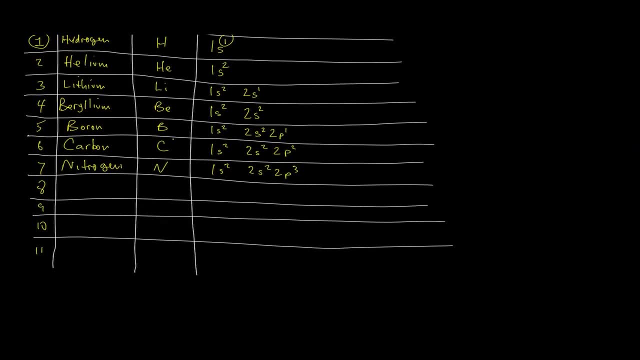 can go all the way up to six if needed. okay, okay, okay. so let's move on to eight, which is so. let's move on to eight, which is so. let's move on to eight, which is oxygen, oxygen symbol, o oxygen symbol, o oxygen symbol, o and. 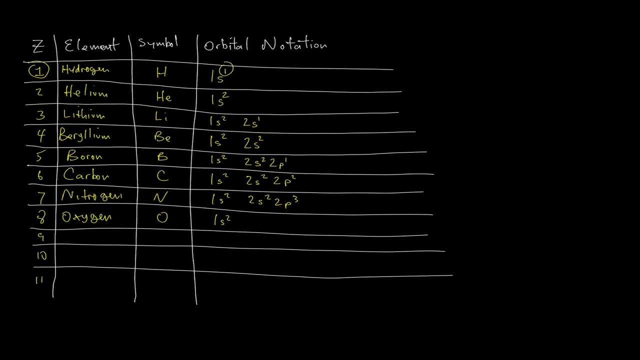 and and the, the, the, as we've called it up here, the orbital as we've called it up here, the orbital as we've called it up here, the orbital notation, notation. notation is one s squared is one s squared is one s squared two s two s squared. 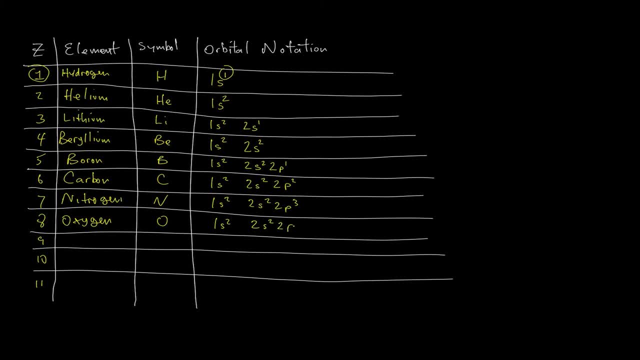 two s squared, squared, squared, squared. two p, two p, two p. this can go up to six. possibly this can go up to six. possibly this can go up to six. possibly for four plus two, for four plus two. for four plus two plus two is eight plus two is eight. 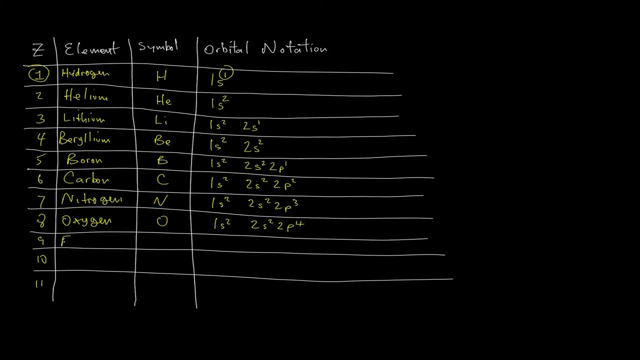 plus two is eight. for oxygen, for oxygen, for oxygen, okay, okay, okay. fluorine is next, fluorine is next, fluorine is next. fluorine is the fluorine. is the fluorine is the symbol f. symbol f. symbol f. we have one s. we have one s. 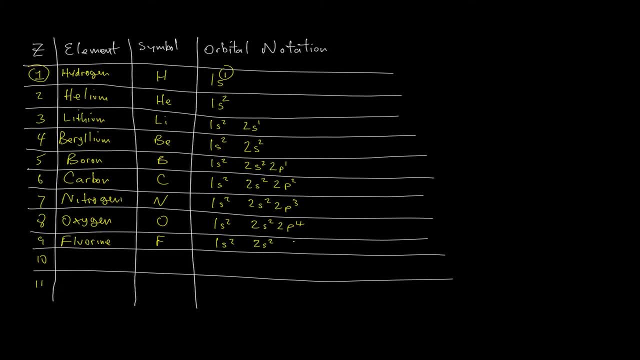 we have one s squared squared. we have one s squared two s, two s squared, two p to the five, two p to the five, two p to the five, predictably, predictably, predictably, okay. five plus two plus two, okay. five plus two plus two, okay. five plus two plus two is nine for fluorine. 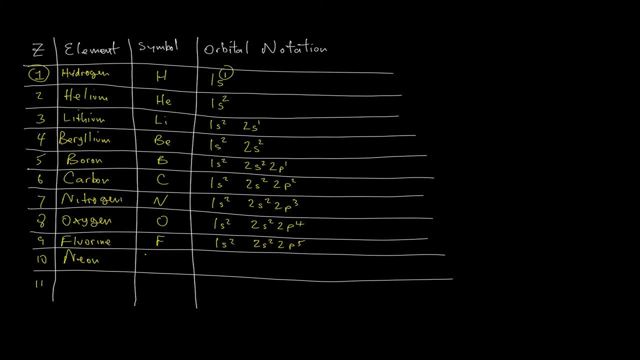 is nine for fluorine, is nine for fluorine. neon, okay, has a atomic number of ten. atomic number of ten. atomic number of ten. symbol is any symbol. is any symbol, is any one s squared? one s squared one s squared two s squared two s squared two p to the six and now this two p. 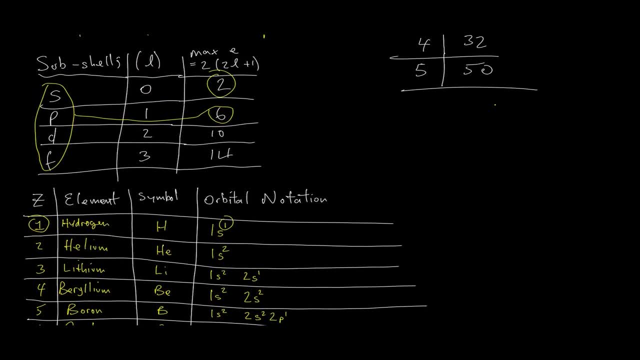 two p to the six, and now this two p, two s squared. two p to the six, and now this two p: shell, shell, shell is full here on neon. okay, this one is is full here on neon. okay, this one is is full here on neon. okay, this one is full. 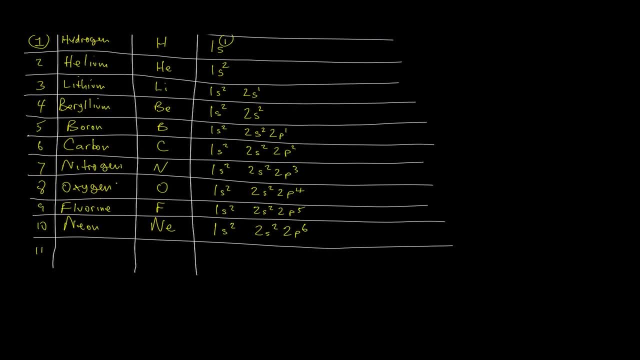 full, full. so we need to move up a shell and this. so we need to move up a shell, and this. so we need to move up a shell, and this is the last one we're going to look at is the last one we're going to look at. 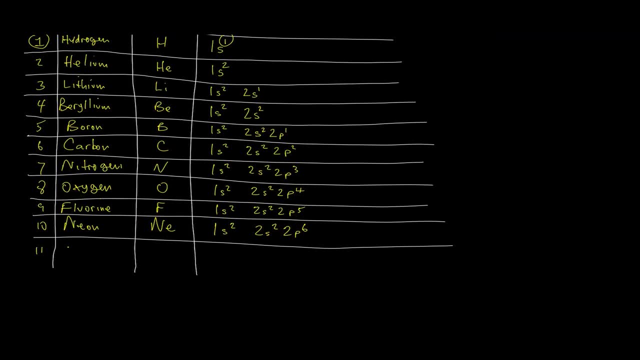 is the last one we're going to look at. i'm going to go through the whole. i'm going to go through the whole. i'm going to go through the whole periodic table for you. you fall asleep. periodic table for you. you fall asleep. periodic table for you. you fall asleep. i'm going to look at sodium. 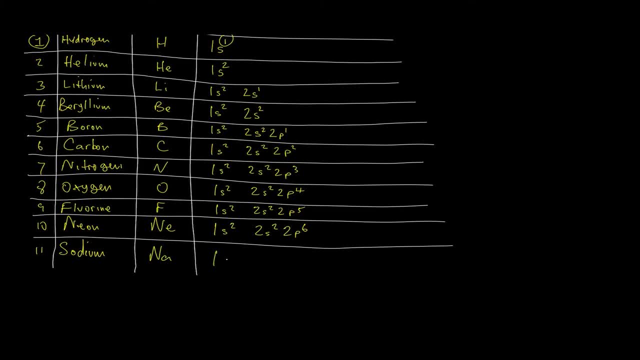 has the symbol in a. we have one s. has the symbol in a. we have one s. has the symbol in a. we have one s. squared, squared, squared. move up a shell. we have two. move up a shell. we have two. move up a shell. we have two s. 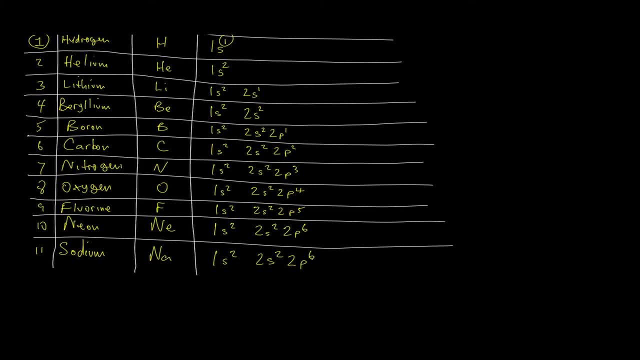 s s squared, squared, squared. two p, two p, two p to the six, to the six, to the six, and then we're going to move up with, and then we're going to move up with, and then we're going to move up with, another shell, another shell. 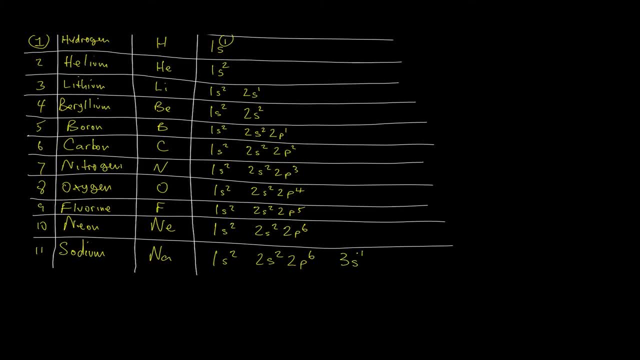 another shell: three, three, three s s s to the one, to the one, to the one. now, then, now, then, now then i want to make something. i want to make something. i want to make something very, very clear here, very, very clear here, very, very clear here. um put the notes over here. 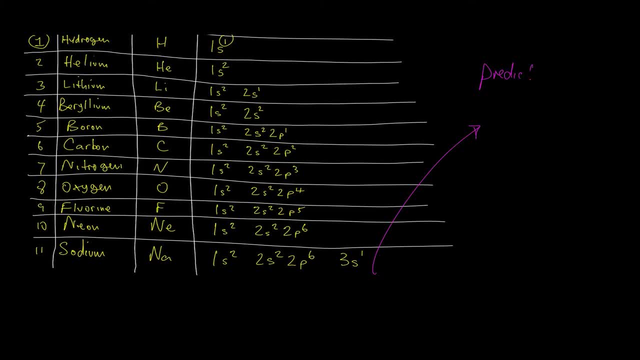 predictable. well, population disappears. it doesn't disappear after sodium, it doesn't disappear after sodium. it doesn't disappear after sodium, it disappears after: i think it's, i think it's, i think it's: z equals 20, z equals 20, z equals 20, calcium, calcium. 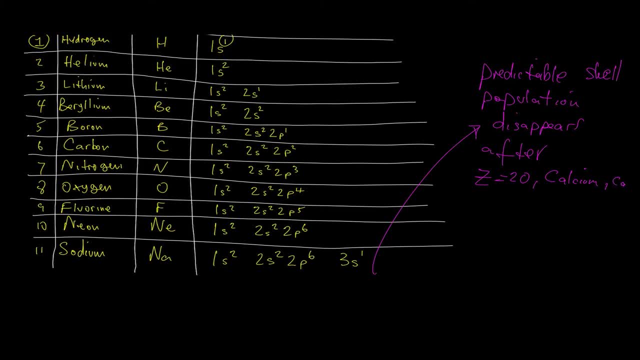 calcium, calcium, which is, which is, which is symbol ca, so up to calcium. symbol ca, so up to calcium. symbol ca, so up to calcium. we can do all this stuff, we can do all this stuff, we can do all this stuff. after that we don't have, after that we don't have. 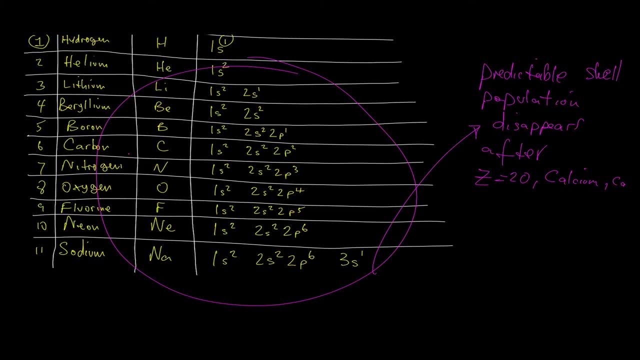 after that we don't have the. the next outer shell isn't the. the next outer shell isn't the. the next outer shell isn't necessarily, necessarily, necessarily the one which is populated next. so the one which is populated next, so the one which is populated next. so it all gets very, very complex. higher. 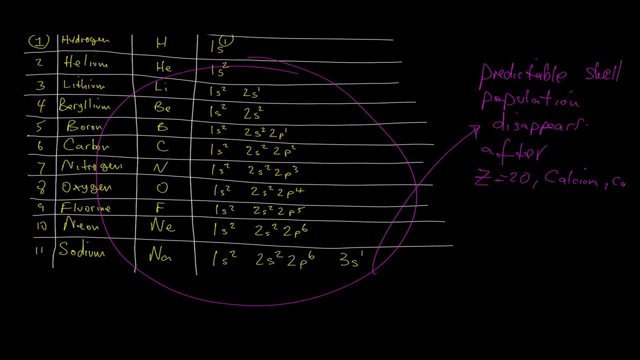 it all gets very, very complex higher. it all gets very, very complex, higher level things, level things, level things you don't need to know about at this, you don't need to know about at this, you don't need to know about at this point, point, point. what i would like to do now is just: 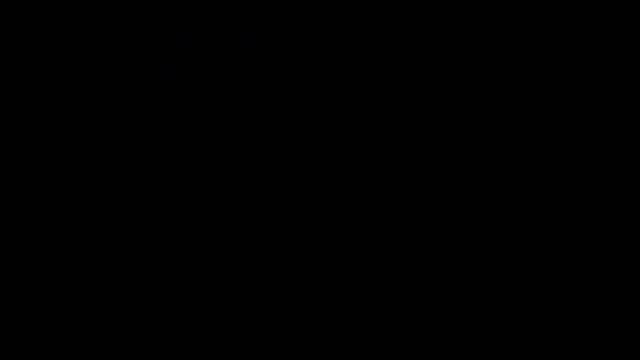 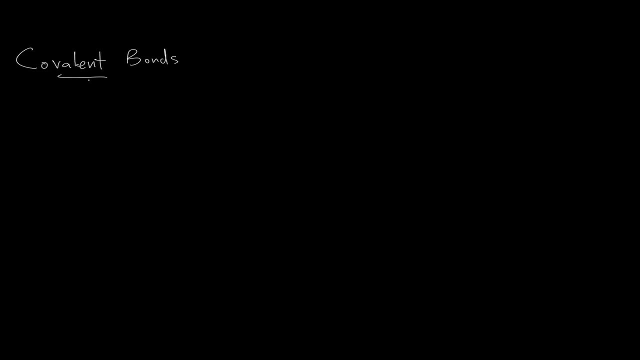 when we say valence, when we say valence, uh, this word valence, we mean, uh, this word valence, we mean, uh, this word valence, we mean the outer, the electrons which occupy the outer, the electrons which occupy the outer, the electrons which occupy the outer shells. they're called valence. 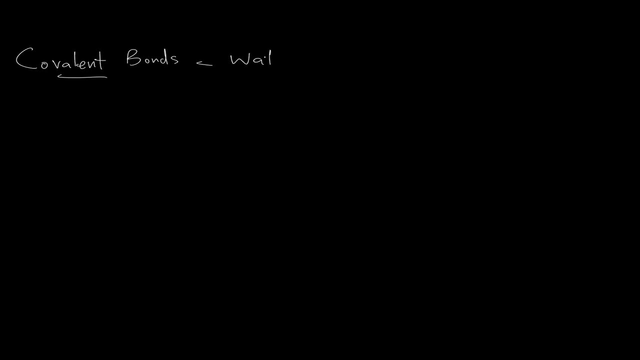 the outer shells, they're called valence, the outer shells, they're called valence electrons. i want to use a electrons. i want to use a electrons. i want to use a specific example. i think specific example. i think specific example. i think we all, we all, we all know and need water, which is h2o. 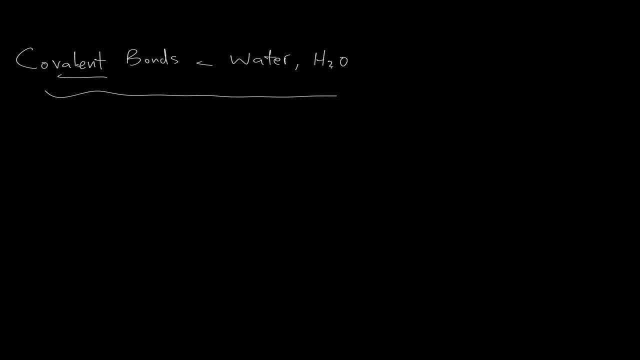 and h2o of course means two hydrogen and h2o of course means two hydrogen and h2o of course means two hydrogen atoms and one oxygen atom that makes up atoms and one oxygen atom that makes up atoms and one oxygen atom that makes up a molecule of water. 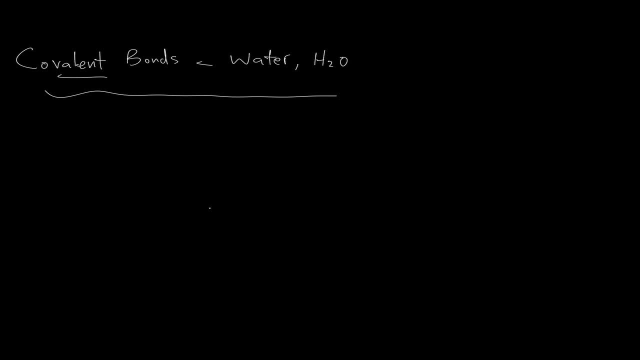 a molecule of water, a molecule of water, so so, so let me finish off here by. let me finish off here by. let me finish off here by drawing a molecule, um, um, um, let me just do an atom first of all. let me just do an atom first of all. 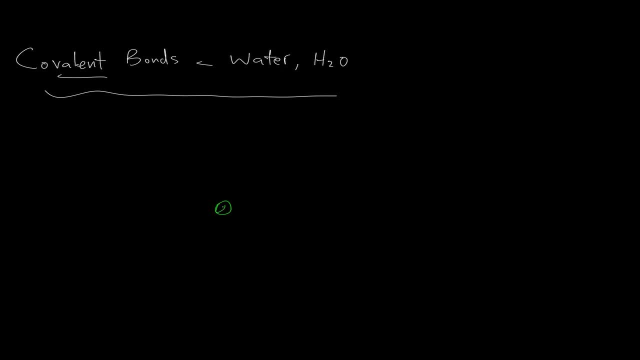 let me just do an atom first of all. maybe i could use green here, so in here, so in here, so in here. we have some oxygen, some oxygen, some oxygen. this is actually an oxygen nucleus. this is actually an oxygen nucleus. this is actually an oxygen nucleus, and 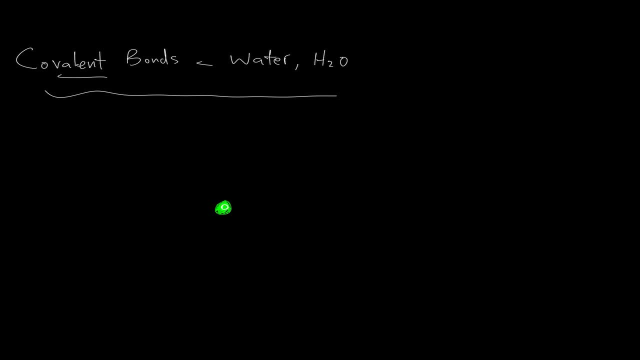 and and maybe i could draw a zip. i know in, maybe i could draw a zip i know in, maybe i could draw a zip i know in there, there, maybe i could draw a zip i know in there. okay, so that is a letter o representing. okay, so that is a letter o representing. 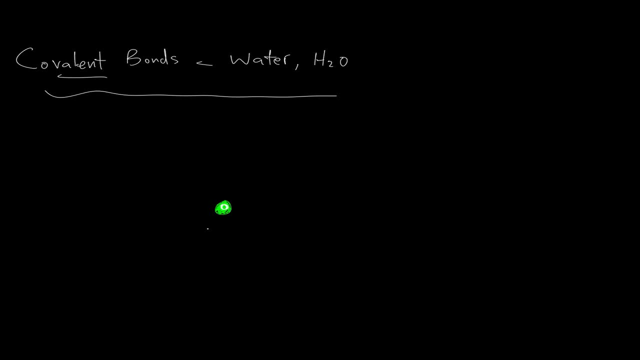 okay, so that is a letter o representing oxygen in that green nucleus. oxygen in that green nucleus, oxygen in that green nucleus. i'm not going to even draw the 1s, i'm not going to even draw the 1s. i'm not going to even draw the 1s subshell here. but what i am going to 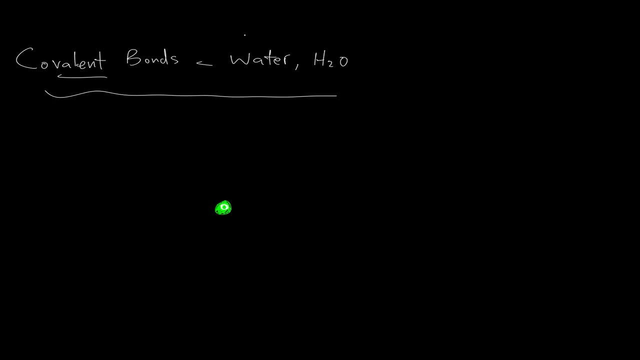 subshell here, but what i am going to subshell here, but what i am going to draw for you, draw for you. draw for you. um, what color can i use here? maybe stick. um, what color can i use here? maybe stick. um, what color can i use here? maybe stick with white. for now i'm going to draw. 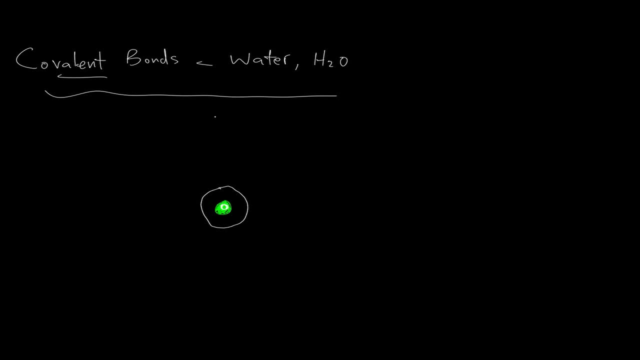 with white. for now, i'm going to draw with white. for now i'm going to draw as best as i can. as best as i can, as best as i can. uh, this is going to be a 2s subshell for oxygen. subshell for oxygen. 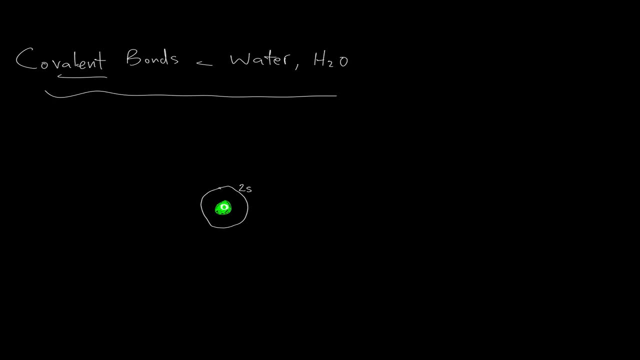 subshell for oxygen and and and maybe the oxygen i can give it, maybe the oxygen i can give it, maybe the oxygen i can give it. blue, blue, blue, dark blue, dark blue, dark blue. maybe not stand out too well give it. maybe not stand out too well give it. 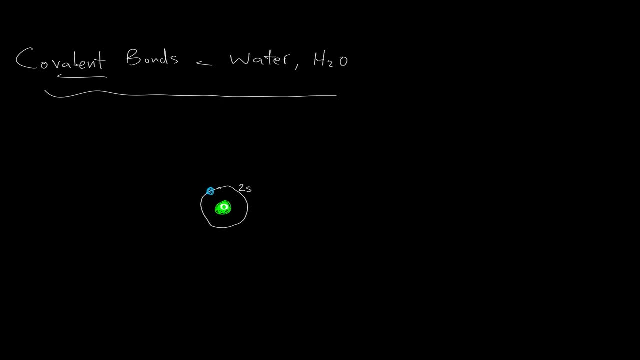 maybe not stand out too well. give it light blue electrons. here we are light blue electrons. here we are light blue electrons. here we are so light blue electrons, so light blue electrons. here we are so light blue electrons for the oxygen. okay, so there's the 2s. 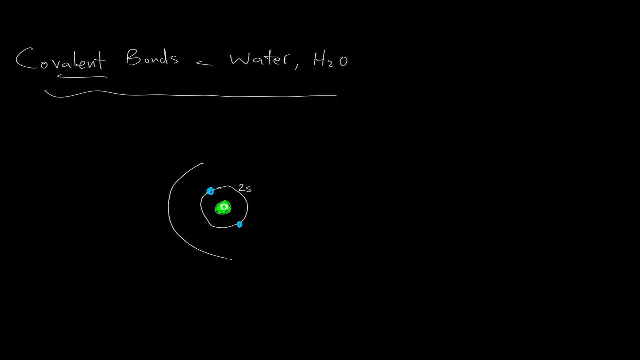 okay, so there's the 2s. okay, so there's the 2s. to draw another, to draw another, to draw another ball bit here, and this is going to be, and this is going to be, and this is going to be: 2p, 2p. 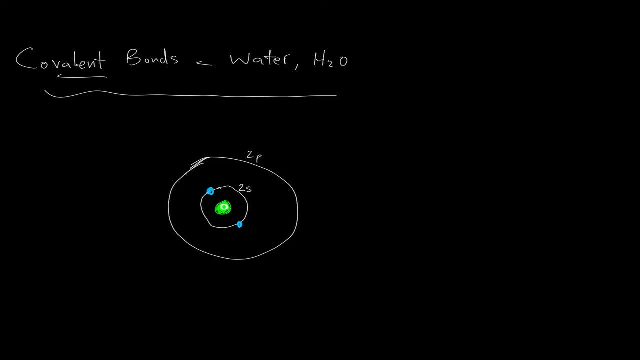 2p. of course, of course, of course it's not a very good join there, but it's not a very good join there. but it's not a very good join there, but never mind. now, now, now in the 2p, in the 2p. 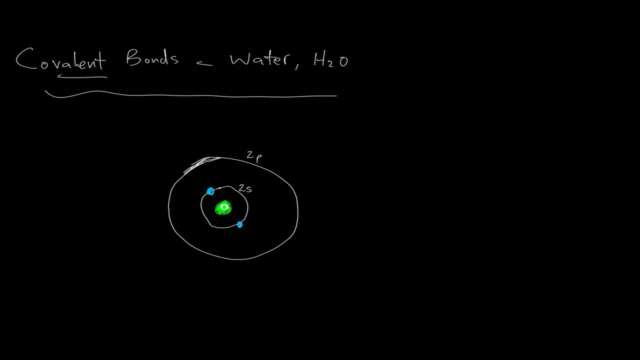 in the 2p for oxygen, for oxygen, for oxygen, let's just go back up and have a look at. let's just go back up and have a look at. let's just go back up and have a look at that table, that table, that table- so oxygen. 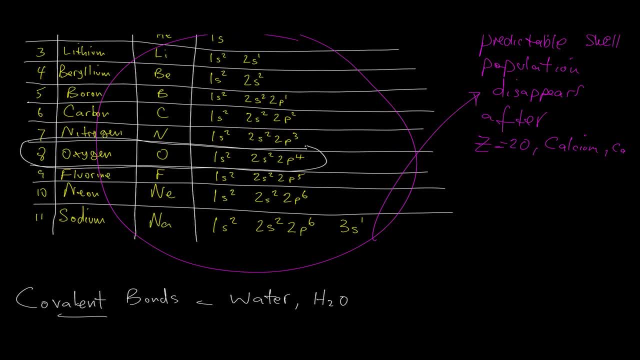 so oxygen, so oxygen, 2p- here we are sort of circled it here. 2p, here we are sort of circled it here. 2p, here we are sort of circled it here for you. so in the second shell it has, so in the second shell it has. 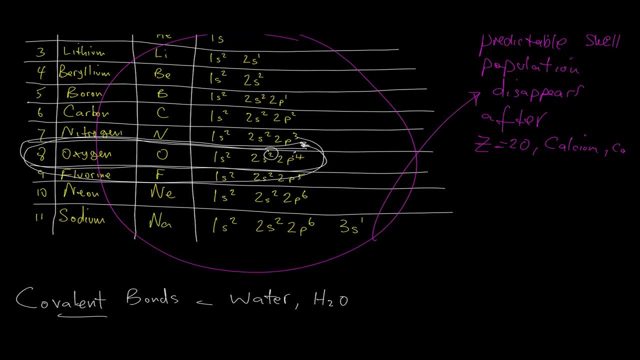 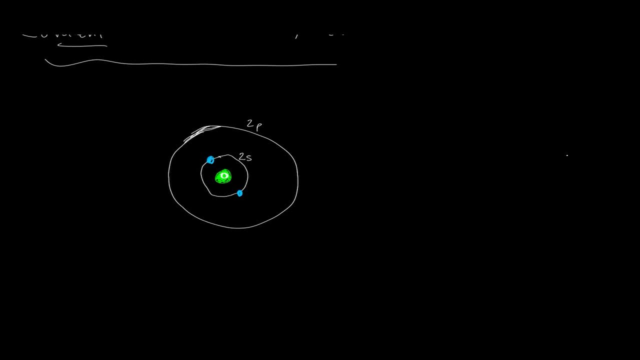 so in the second shell, it has six electrons here, six electrons here, six electrons here, that two and that four, that two and that four, that two and that four gives us six, gives us six, gives us six, okay, okay, okay. well, here's two of them here in the 2s. 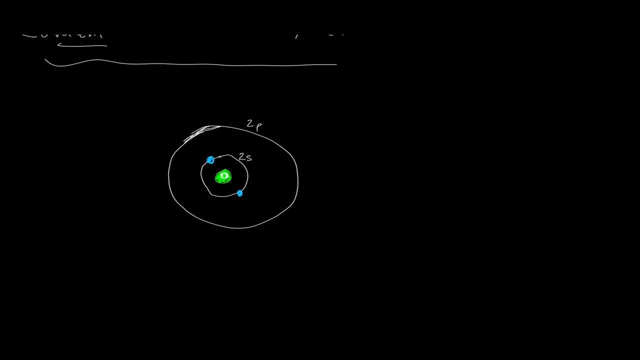 well, here's two of them here in the 2s. well, here's two of them here in the 2s. so therefore, so, therefore, so, therefore, 2p must have change color again. let's go back to that. change color again. let's go back to that. 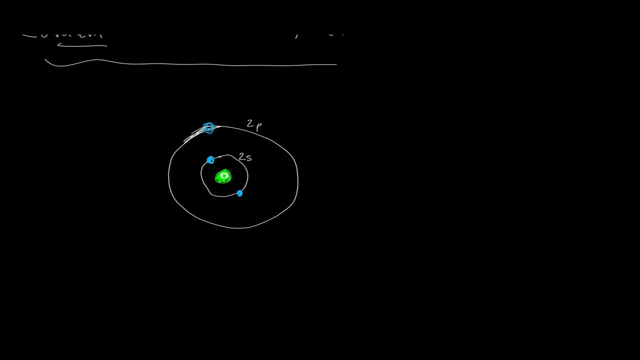 change color again. let's go back to that blue, blue, blue, 2p. it should all be the same size by 2p. it should all be the same size by 2p. it should all be the same size. by the way, these electrons, of course. 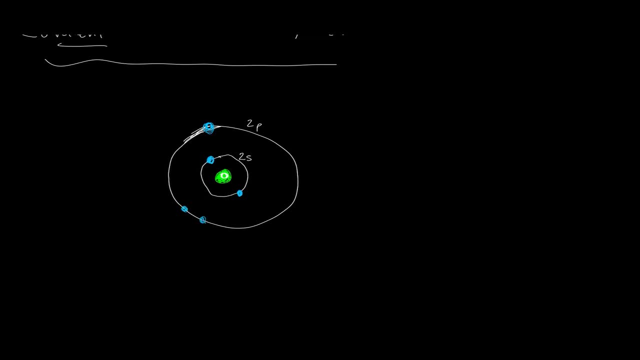 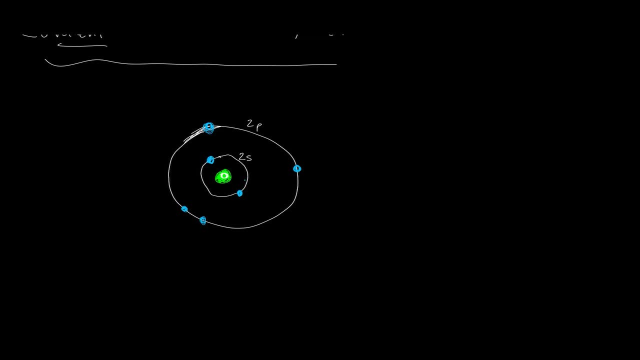 in blue, here we have the six electrons. in blue, here we have the six electrons which occupy, which occupy, which occupy: uh, shell number two, uh, shell number two, uh, shell number two for oxygen, for oxygen, for oxygen, these two here, we call alone her. we call alone her. 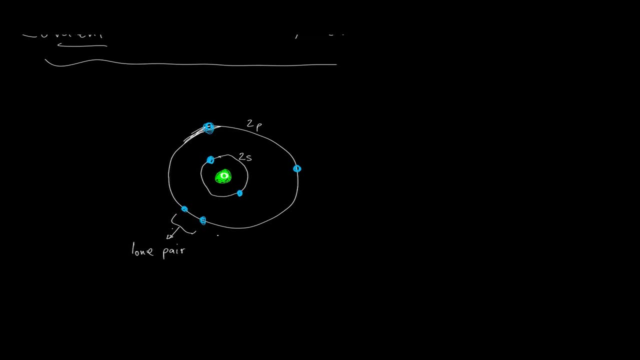 we call alone her, because they're not going to be, because they're not going to be, because they're not going to be, associated or bonded. associated or bonded, associated or bonded through the um, through the um, through the um. electron orbits of anything else. electron orbits of anything else. 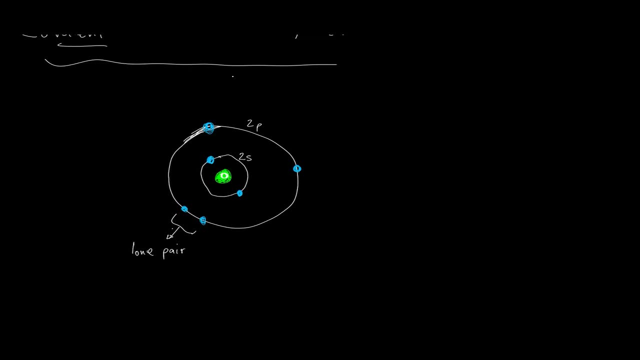 electron orbits, of anything else, for the time being, at least for the time being, at least for the time being, at least what i'm going to do. what i'm going to do, what i'm going to do is in white. i'm going to draw here very bad circle. 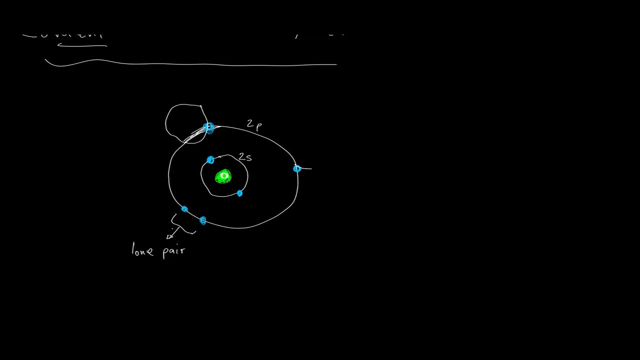 very bad circle, very bad circle. um, hopefully this one can be a little bit, hopefully this one can be a little bit, hopefully this one can be a little bit better for you, better for you, better for you. you get the idea, okay, you get the idea. okay, you get the idea. okay. so there's a circle. 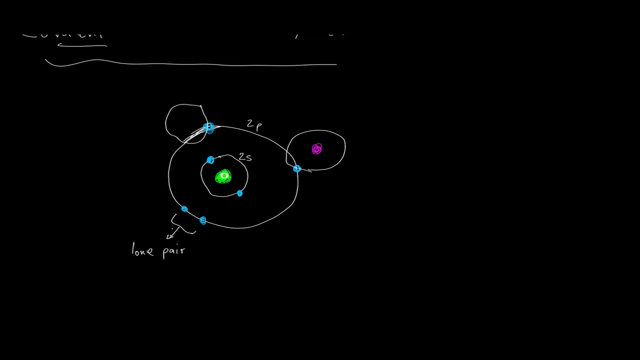 so there's a circle. so there's a circle. this thing here is going to be: when i fill it in, it's going to be when i fill it in, it's going to be: when i fill it in, it's going to be hydrogen, hydrogen, hydrogen. so this is going to be. 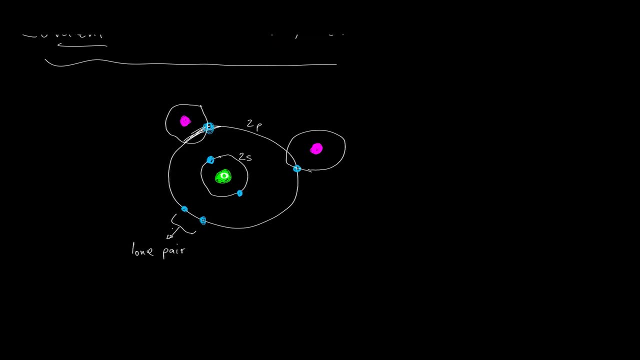 so this is going to be. so this is going to be a couple of hydrogen, a couple of hydrogen, a couple of hydrogen atoms put h in there h atoms put h in there. h atoms put h in there, h and a h and a h and a h. um, possibly. what color have i got? 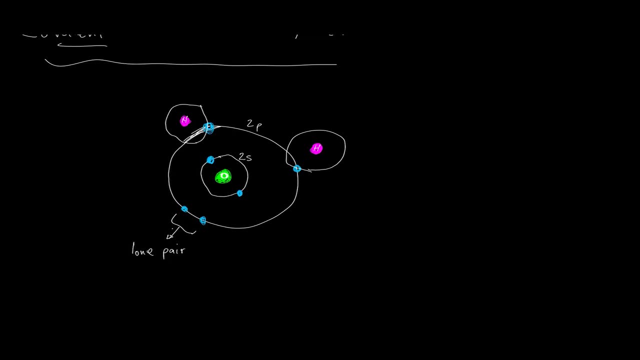 um, possibly, what color have i got? um, possibly, what color have i got? square here yellow. square here yellow. square here yellow. i'll put the hydrogen's um electron in. i'll put the hydrogen's um electron in. i'll put the hydrogen's um electron in as yellow, shall i? 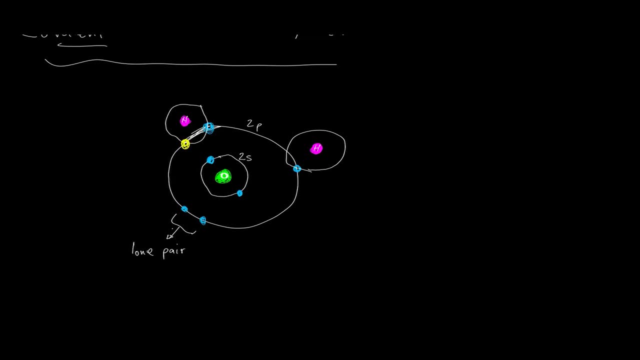 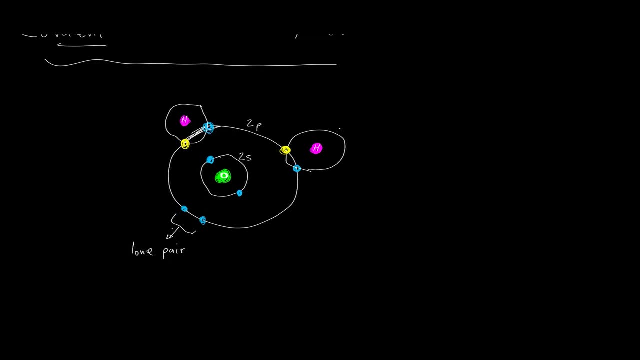 and can you see, possibly, what's happened, and can you see possibly what's happened here, here, here? well, let me make a note of this one. well, let me make a note of this one. well, let me make a note of this one. so, in this one, so in this one. 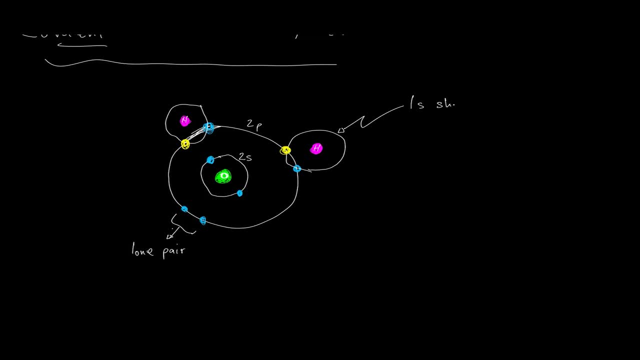 so in this one for hydrogen, the 1s shell of hydrogen, of hydrogen, of hydrogen, appears. this is the important bit appears. this is the important bit appears, this is the important bit appears filled with two electrons, with two electrons with two electrons. okay, okay, okay. standard hydrogen atom, of course, only has 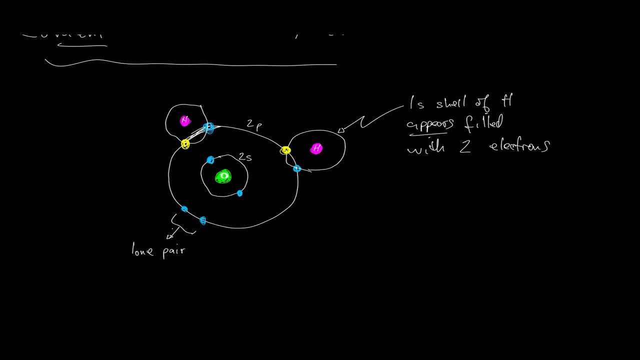 standard hydrogen atom. of course only has standard hydrogen atom. of course only has one, however one, however one. however, it's one s shell can accommodate two. it's one s shell can accommodate two. it's one s shell can accommodate two, and we have a more stable situation. 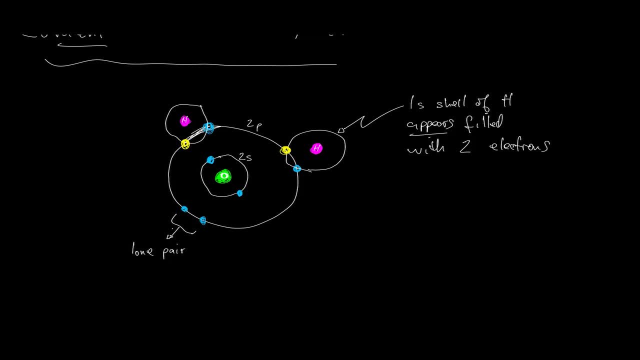 and we have a more stable situation. and we have a more stable situation happening, happening, happening, when, when, when shells are filled, or some sharing goes on, shells are filled, or some sharing goes on, shells are filled, or some sharing goes on, and that fills the shells, okay, finally, 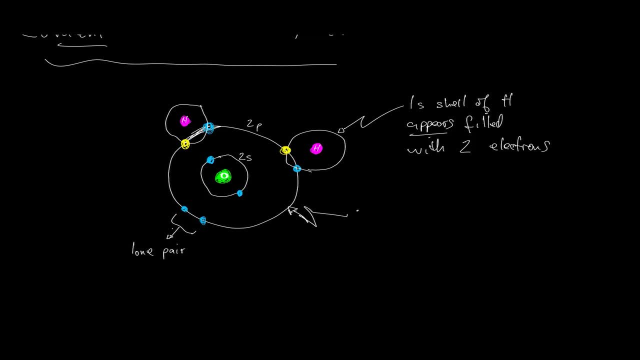 and that fills the shells, okay, finally, and that fills the shells, okay, finally. we'll look here because this is, we'll look here because this is. we'll look here because this is happening twice, happening twice, happening twice. this is here, we have the 2p. this is here, we have the 2p. 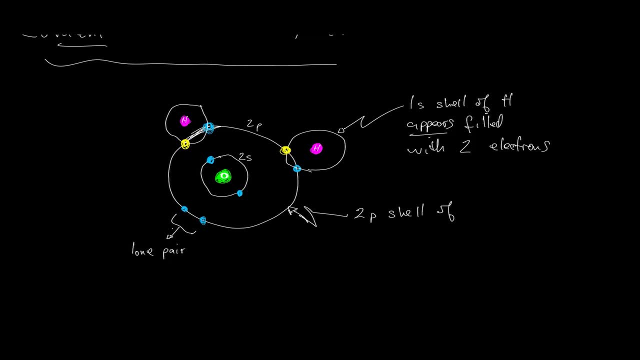 this is here we have the 2p shell, or subshell of oxygen appears filled with its maximum of six electrons, even though in reality, of six electrons, even though in reality, of six electrons, even though in reality it only has four. it only has four, it only has four. so this is what the sharing does, the 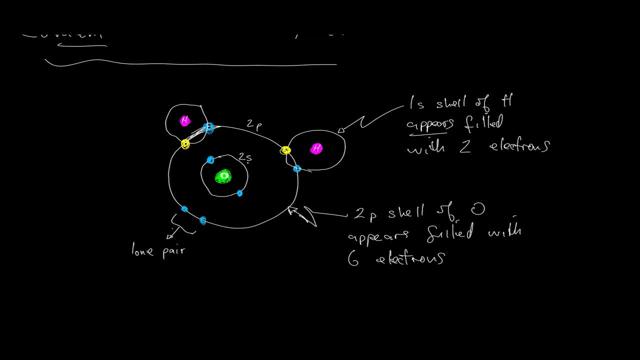 so this is what the sharing does, the. so this is what the sharing does. the sharing sees two advantages. sharing sees two advantages. sharing sees two advantages, and that's why we have um and that's why we have um and that's why we have um: lots of bonding between two hydrogens and 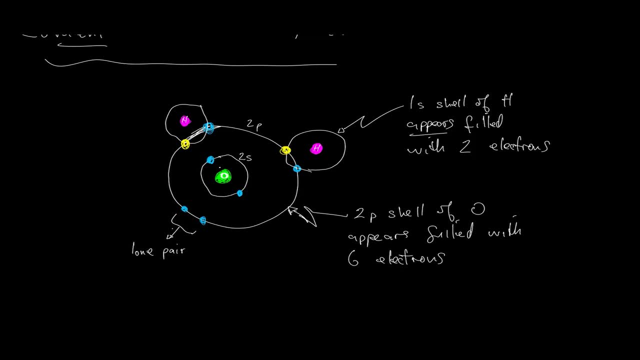 lots of bonding between two hydrogens and lots of bonding between two hydrogens and an oxygen, and that's the reason why an oxygen, and that's the reason why an oxygen, and that's the reason why water is so abundant. water is so abundant. water is so abundant. okay, there's a lot more to bonding and